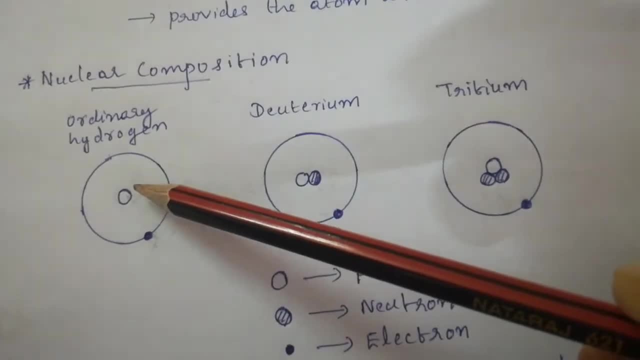 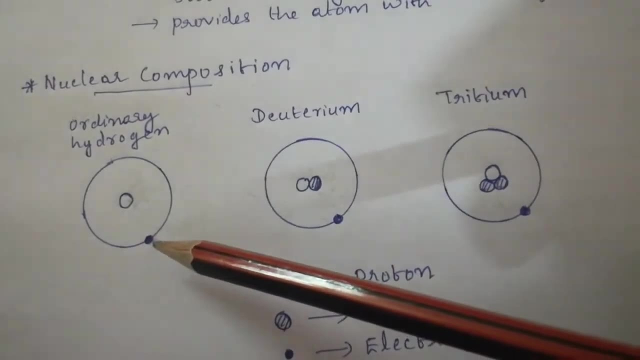 Neutron is uncharged and its mass is slightly greater than that of the proton. Jointly or collectively, these neutrons and protons are uncharged. These neutrons are called nucleons. Now let's move on to the atomic number of an element. 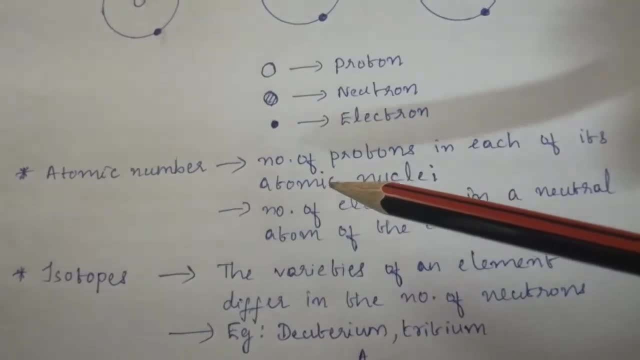 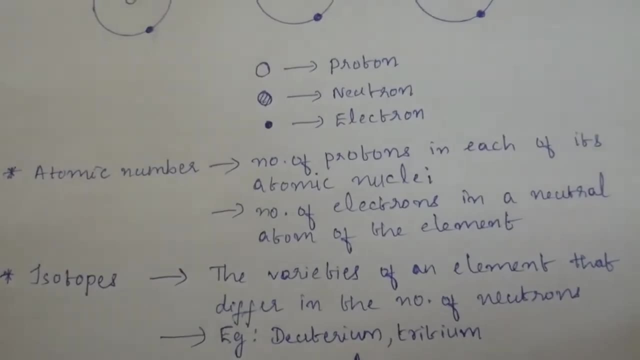 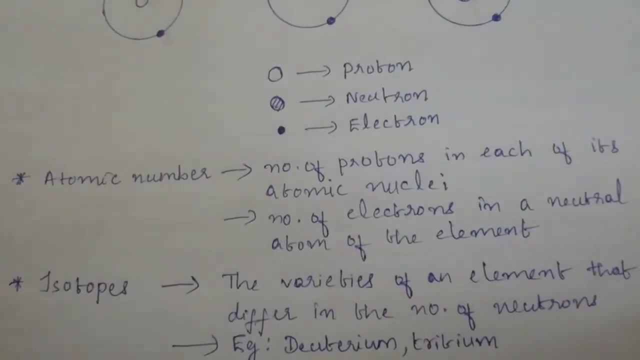 The atomic number of an element is the number of protons in each of its atomic nuclei. This is same as the number of electrons in a neutral atom of the element. For example, atomic number of hydrogen is 1 and that of helium is 2 and that of lithium is 3.. 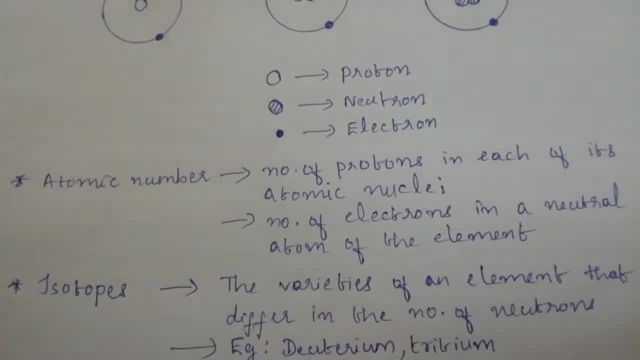 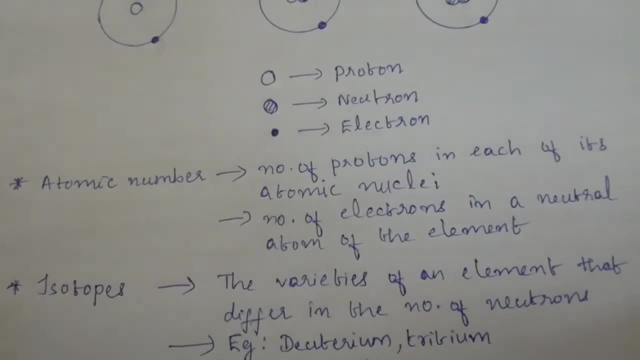 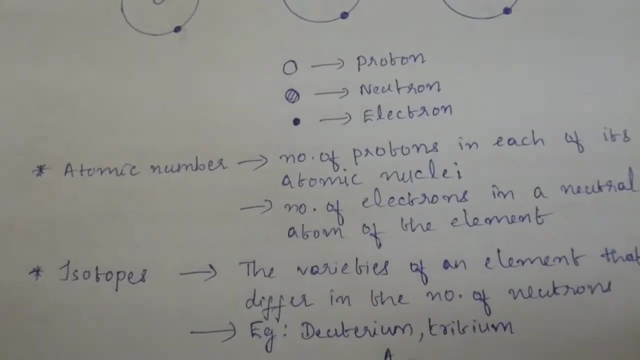 Also, the atomic number of uranium is 92.. Now, 99.9% of hydrogen nuclei are single protons, and a few contain one neutron and a very few contain two neutrons along with the proton. Now, what are isotopes? 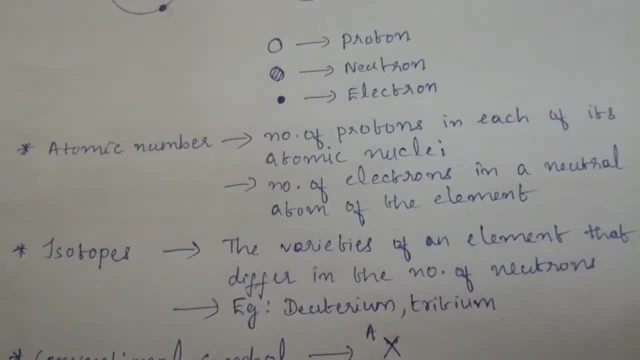 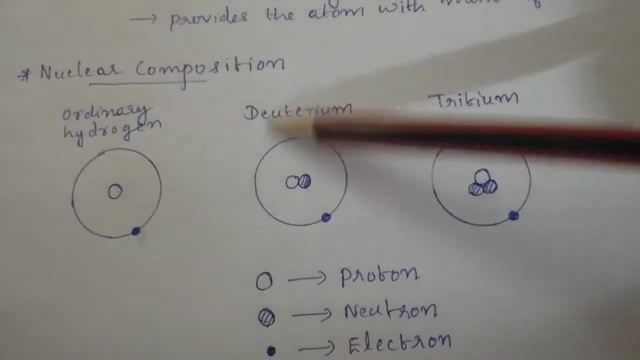 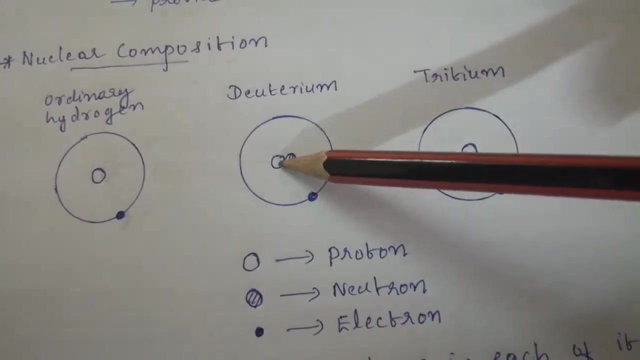 Isotopes are the varieties of an element that differ in the number of neutrons. Now, there are two hydrogen isotopes: One is deuterium, which is shown here, and the other one is tritium. Now, deuterium consists of one proton and one neutron, and tritium consists of one proton and two neutrons. 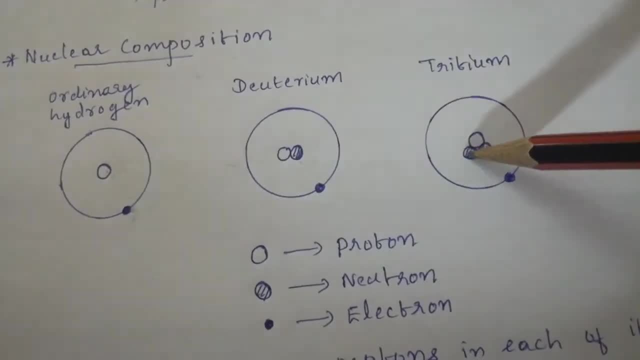 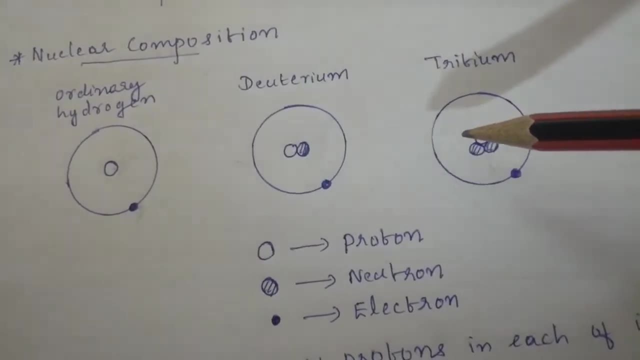 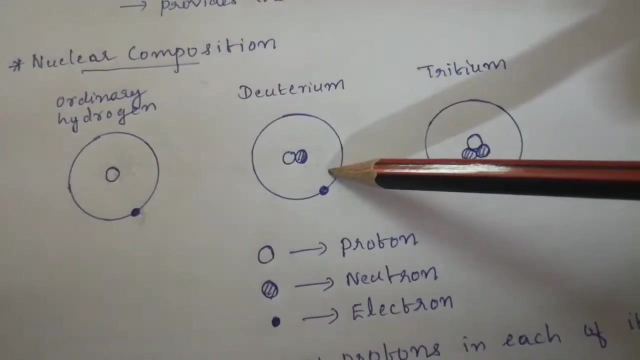 Now deuterium is a stable isotope and tritium is radioactive and it eventually changes into a helium isotope. Now we all have heard about heavy water. right, In heavy water, instead of ordinary hydrogen atom, deuterium atom combines with the oxygen atoms. 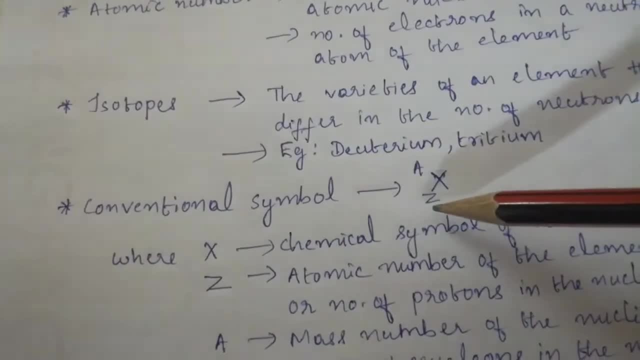 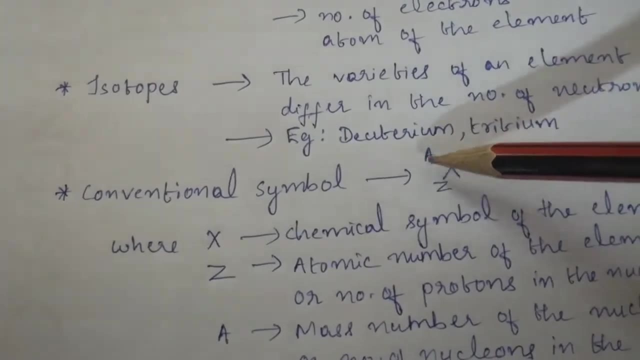 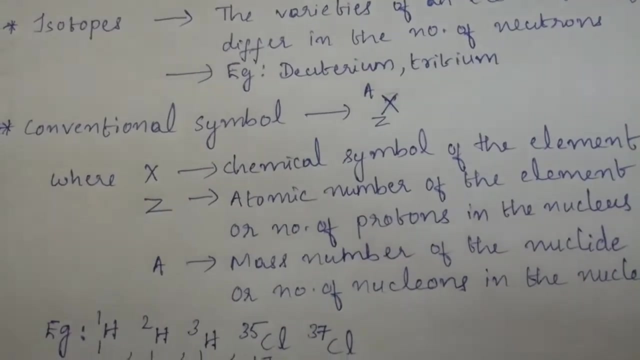 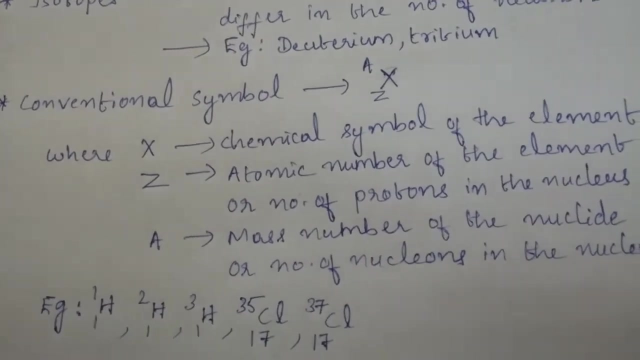 Now the conventional symbol for a nucleoid or nuclear species is given by this, That is, XZA, where X is the chemical symbol of the element and Z is the atomic number of the element, or number of protons in the nucleus, and A is the mass number of the nucleoid, or number of nucleons in the nucleus. 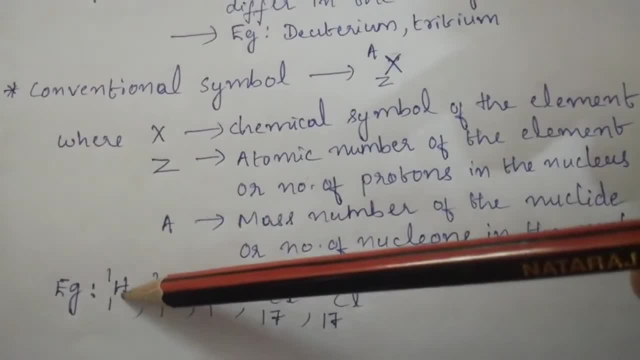 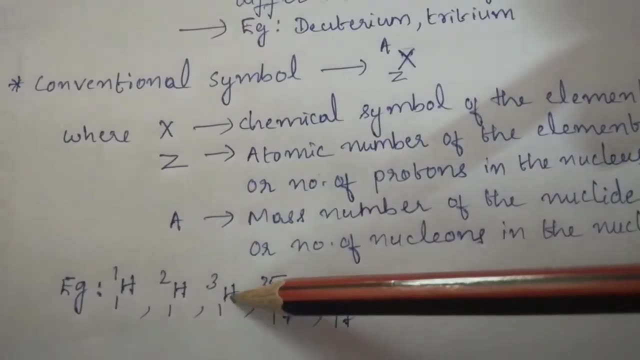 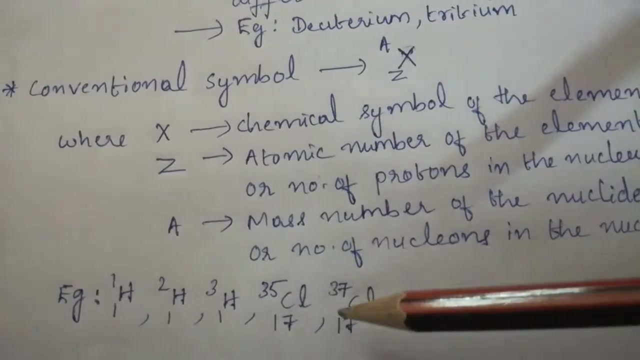 Examples are shown here. Ordinary hydrogen atom is represented as 1H1 and deuterium is 1H2 and tritium is 1H3.. Now what about chlorine? Chlorine has two isotopes, namely chlorine 35 and chlorine 37..